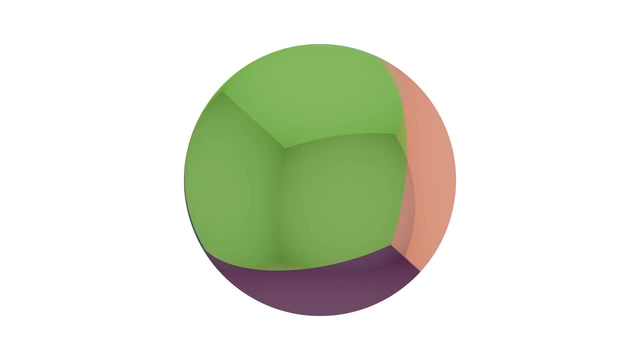 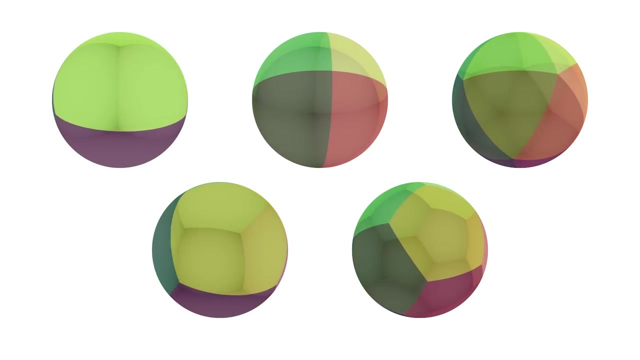 three triangles, four triangles or five triangles? And just a reminder, all these edges are straight lines. Everything lives on that two-dimensional shell and there's no third dimension to curve into. We're only using the two-dimensional shell that forms a triangle. It's just that, with a perfect decline of a speed, 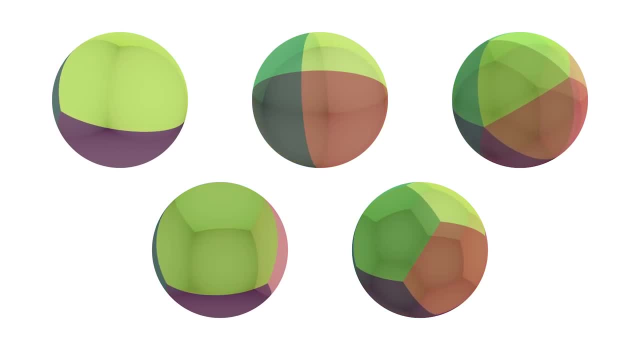 We only use the two-dimensional shell that forms a triangle. It's just that, with a perfect decline of a speed, it to help visualize the space. So now let's move on to hyperbolic space. The theme you'll see for the rest of the video is that, for everything weird about, 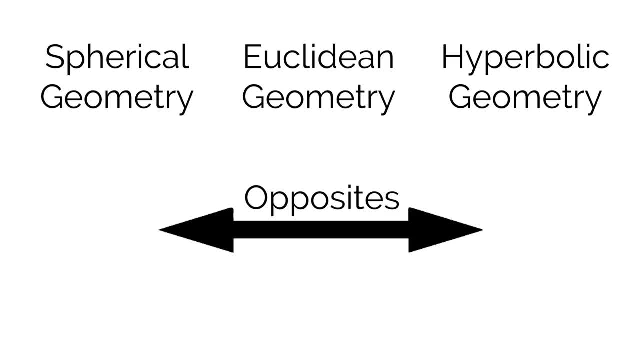 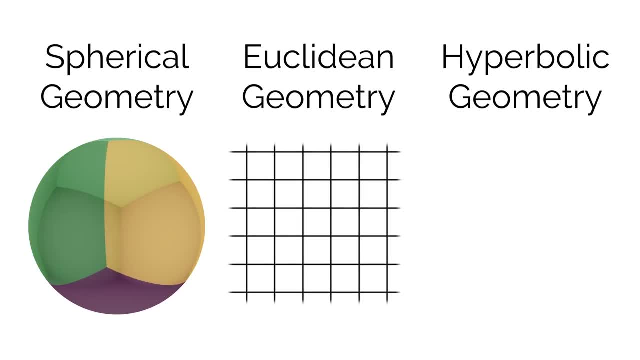 spherical geometry. the opposite is true for hyperbolic geometry, For example. you just saw that we could have fewer squares around each vertex compared to Euclidean space. So in hyperbolic space we can have more, But how could you cram in another square? Well, maybe we can do the same trick as the sphere and just 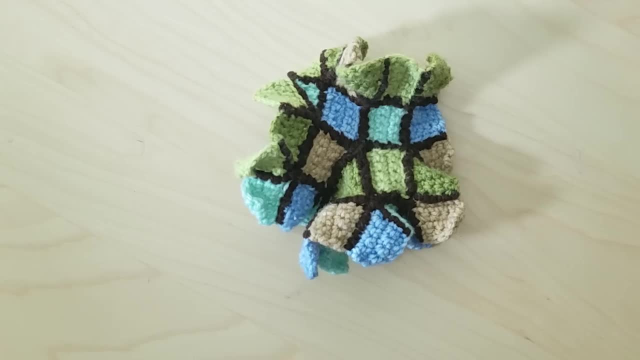 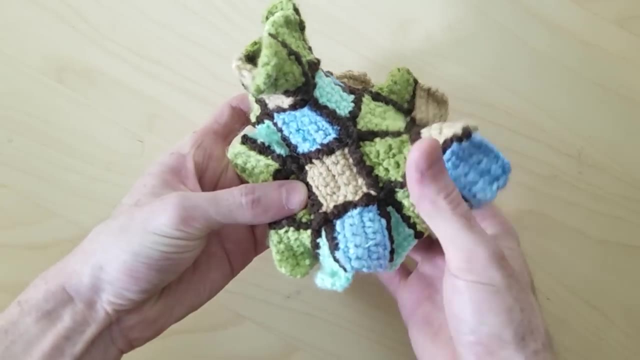 bring it out into the third dimension. We can, and here's how it looks. This is hyperbolic crochet, courtesy of Mrs Parade. You can see how five squares meet at every vertex now, but it's still hard to visualize everything, even with a 3D. 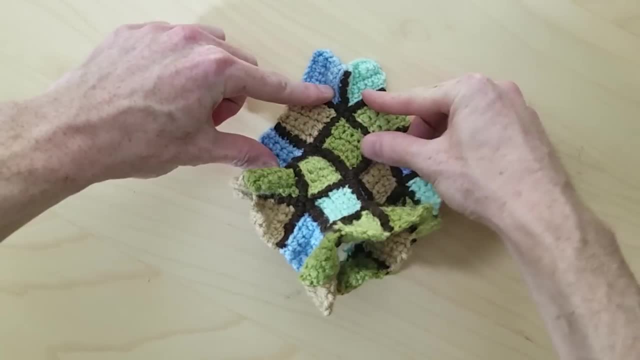 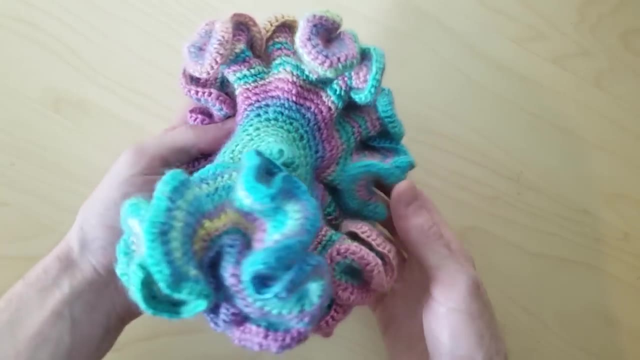 model, because if you try to flatten it in one area, everywhere else starts curving. It's impossible to see it all at once and it gets even worse as we look at bigger and bigger pieces of the hyperbolic plane, Though it does give you. 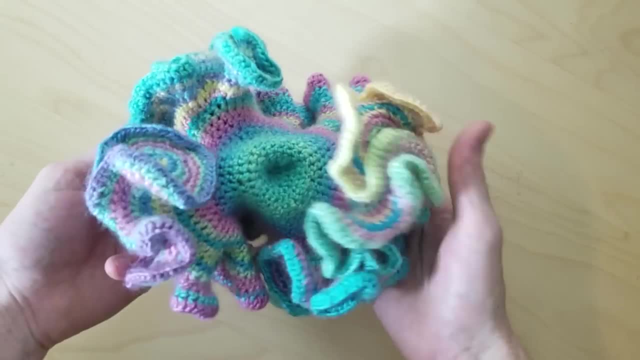 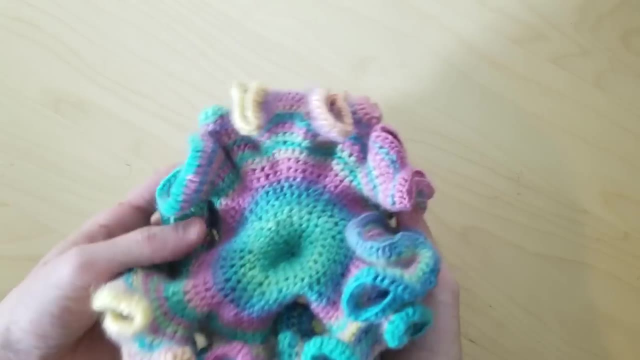 a sense of reality. And don't forget, these are all still two-dimensional geometries, that we're using an extra dimension to help visualize. If we want to go up to 3D spaces, then good luck trying to visualize the 3D surface of a 4D. 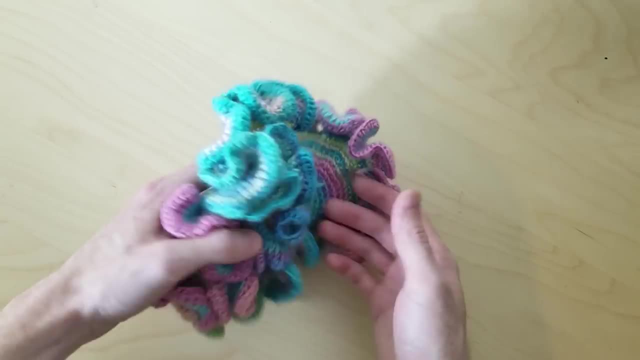 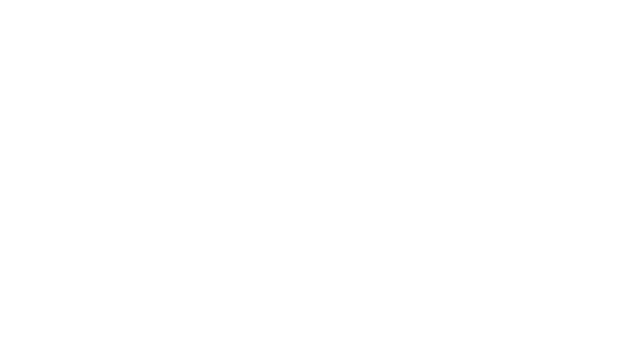 hypersphere, or whatever this mess would look like in four dimensions. In order to make any sense of things at this point, we're going to need a different way to visualize the hyperbolic plane. The trick we're going to use is projection. You're. 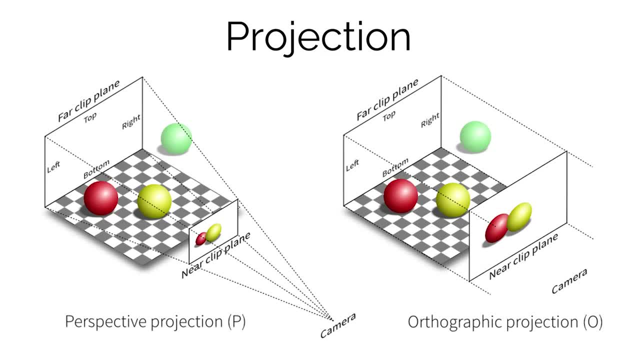 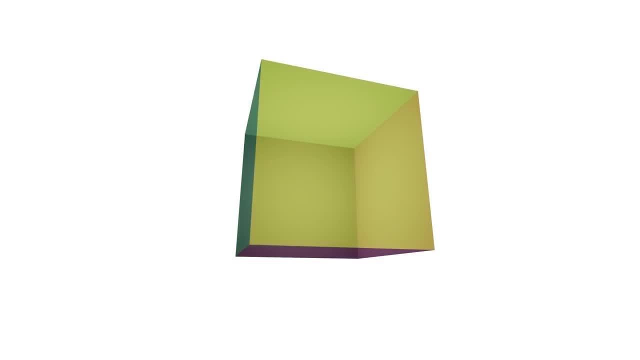 probably familiar with the hyperbolic plane and you're probably familiar with the 3D projection that is, taking a 3D object and projecting it to your eyeball or a screen. After all, you're looking at this cube on your 2D screen, but you still perceive it. 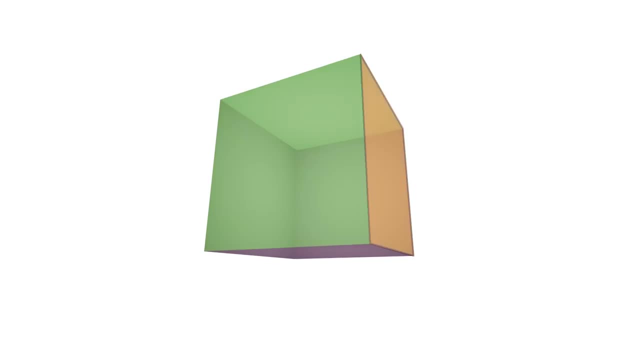 as 3D, even though we've completely distorted it. I mean, this is supposed to be a square, but look at all these angles. Is the cube warped? Of course not. it's just that projected angles and distances can change depending on where you look at it from and what projection. 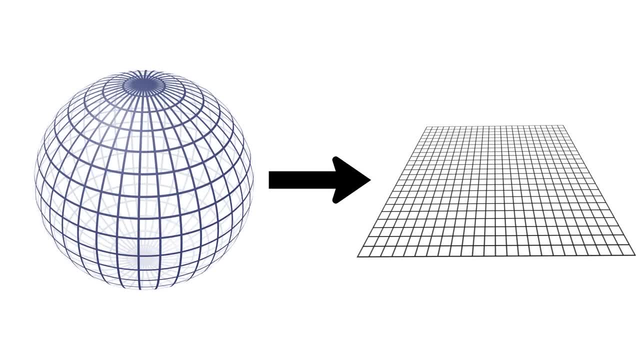 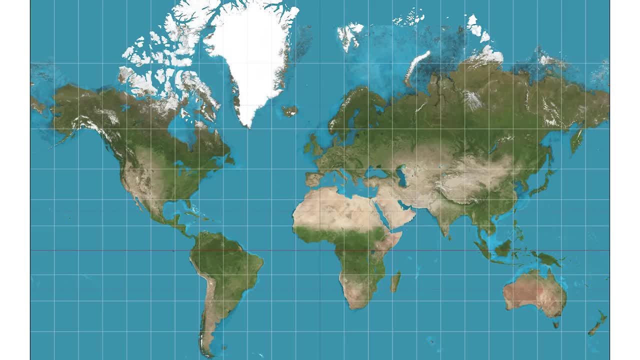 you use. Similarly, we can project a curved geometry to a flat one or a vertical one, or vice versa. You're probably familiar with the Mercator projection for a sphere but, as you can tell, it introduces distortions. Greenland and Africa look about the same size. 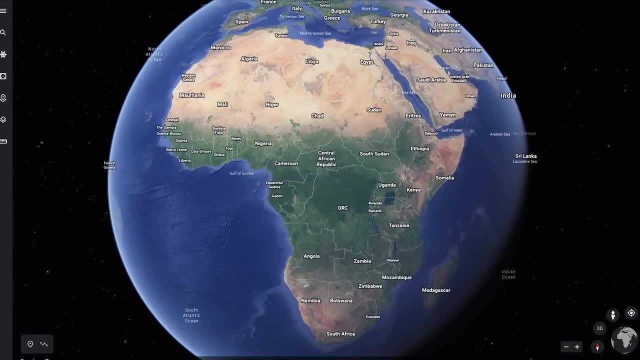 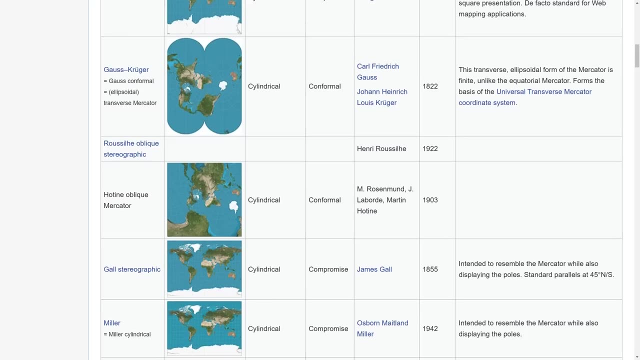 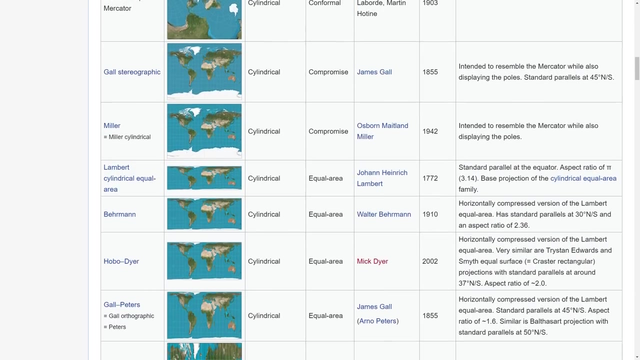 here, but Africa is actually 14 times larger. Unfortunately, it's impossible to map a sphere to a plane without introducing distortion, and that's why there's hundreds of different projections, because either distances, angles, areas or shapes will get distorted, and which? 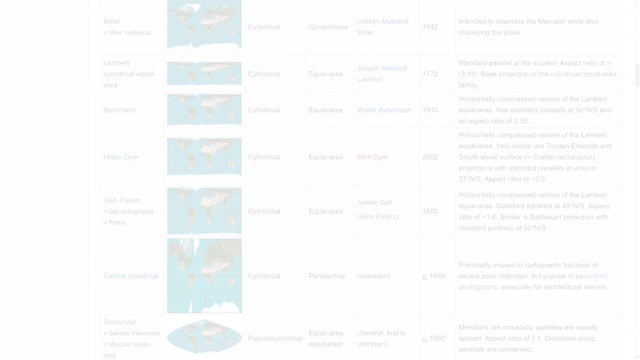 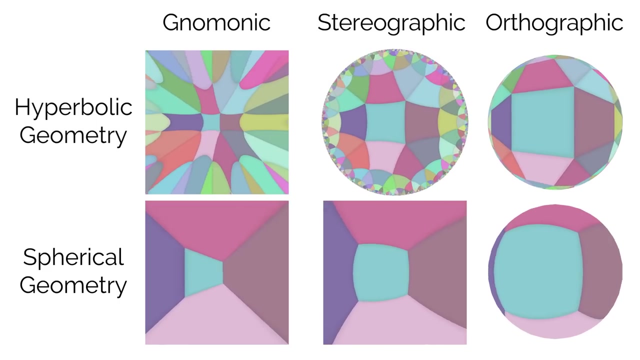 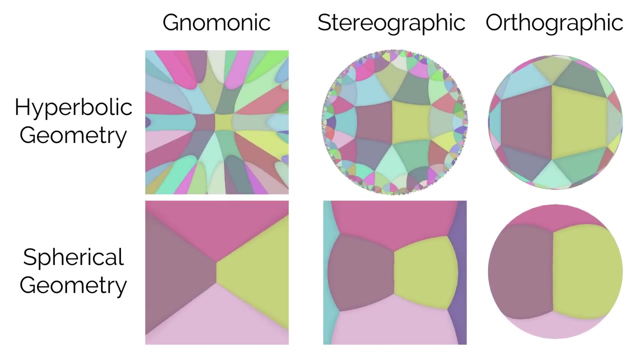 compromise you want depends on the object. We're going to use the 3D projection to see how it works. I'm going to be focusing on a very useful type of projection: stereographic projection. I'm not going to go into too much detail on this because Henry Segerman 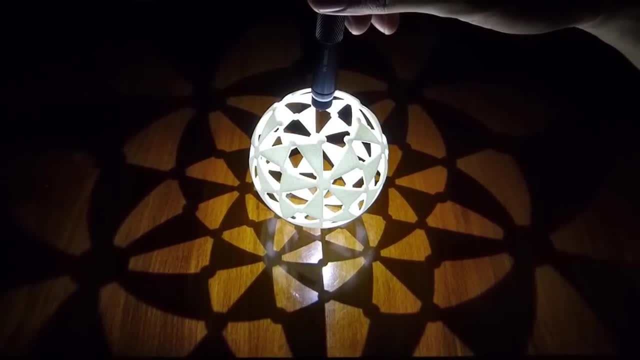 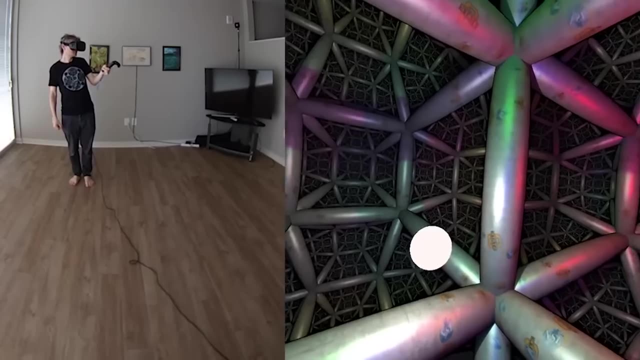 already has a great video that shows how all these projections work on the spherical and hyperbolic planes using just light and shadows. It's super cool, so definitely check out that video. Also, I want to thank Henry, because he's been a huge help with Hyperbolica. I. 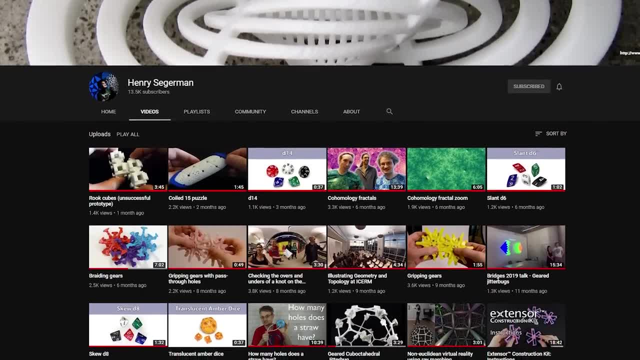 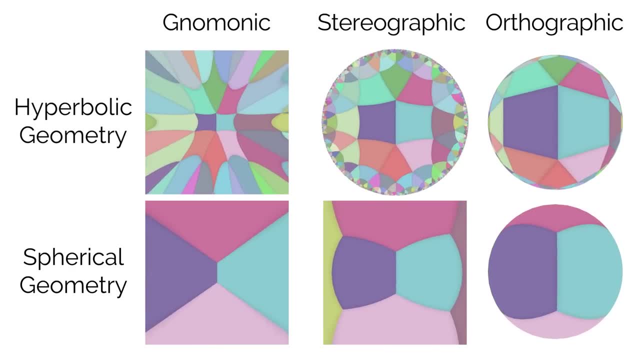 really don't think I could have done it without him, and his YouTube channel is totally underrated, so go subscribe if you like things like this. Okay, now that we have a better way to visualize spherical and hyperbolic space, we can start. 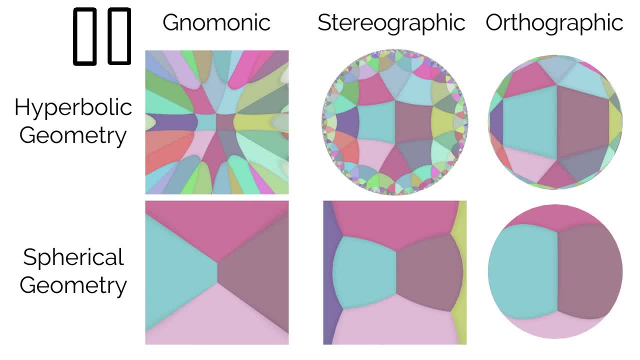 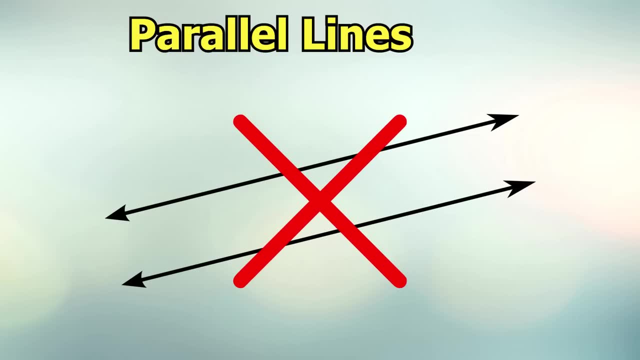 making some sense of its weird properties. But first I have to talk about parallel universa- I mean lines. Parallel lines, They don't exist in spherical space. Any pair of spherical and hyperbolic lines will always converge and intersect eventually. so the whole concept. 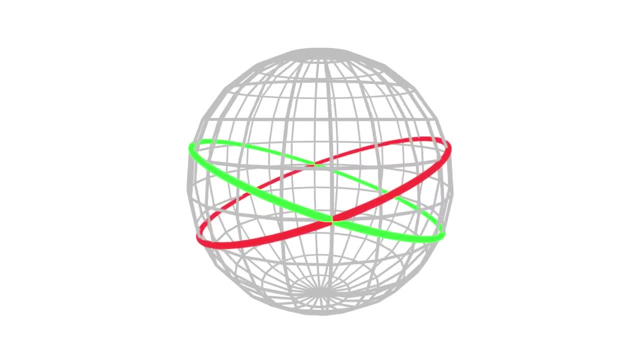 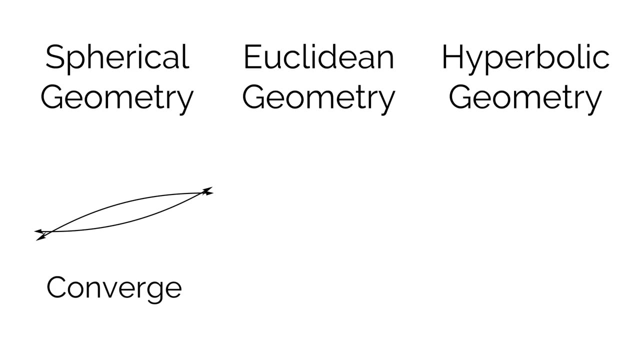 of two things being parallel is not a global property anymore. It's a local phenomena that only exist at a point on the line. And remember how everything hyperbolic is the opposite of spherical. Well, in hyperbolic, space, lines will always diverge. Remember. 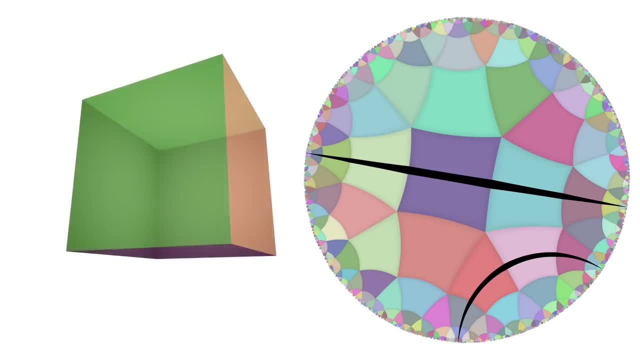 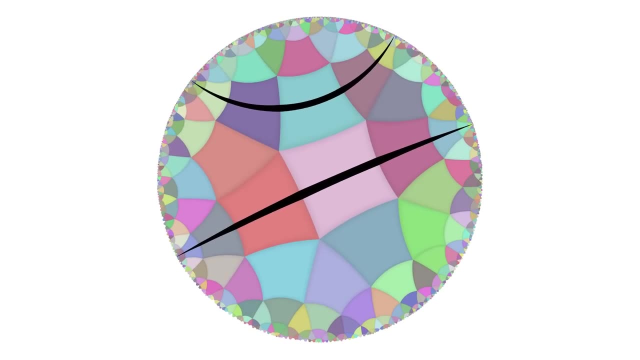 both of these are straight lines, just like how. this is actually a square. It just depends on what angle you're looking at it from. so walking over to the other line will shift your perspective. to see it was straight the whole time. Speaking of walking, let's take a walk on the sphere. Let's walk up one tile right. 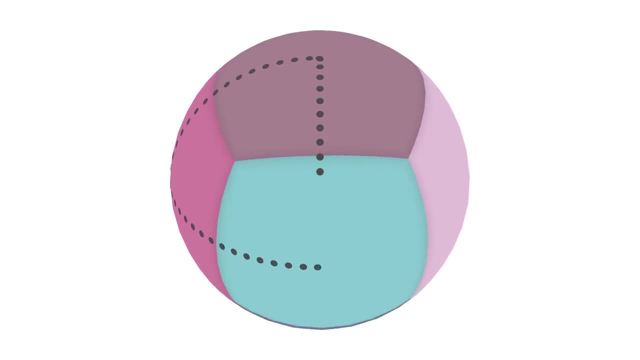 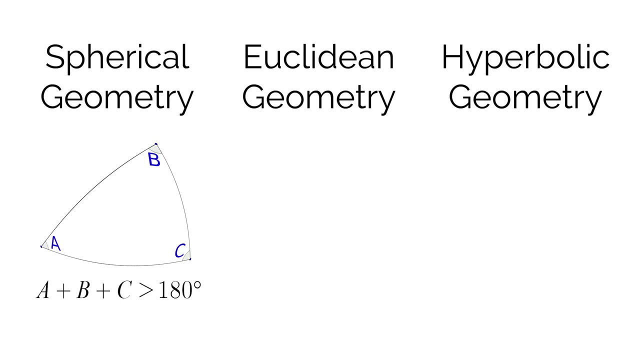 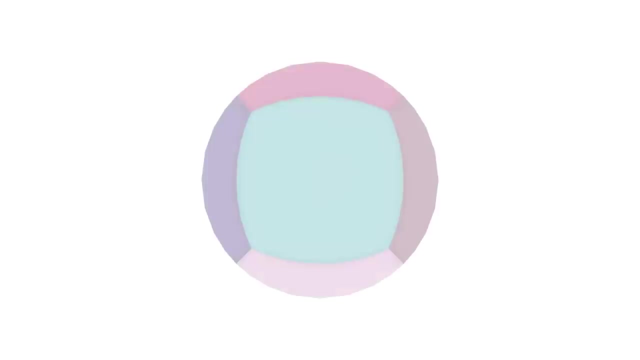 one tile and then down one tile. We're back where we started and we just walked around a triangle with three right angles. In Euclidean space, a triangle's angles have to sum to 180 degrees, but in spherical space it's always larger. 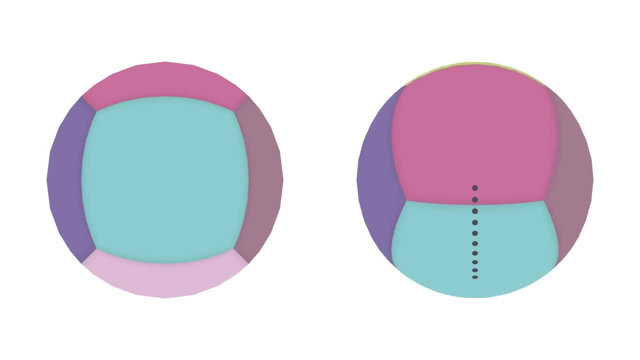 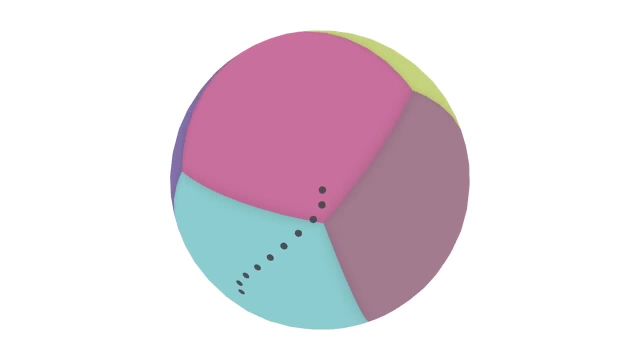 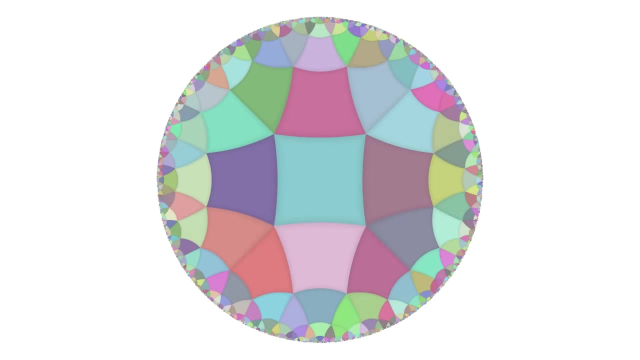 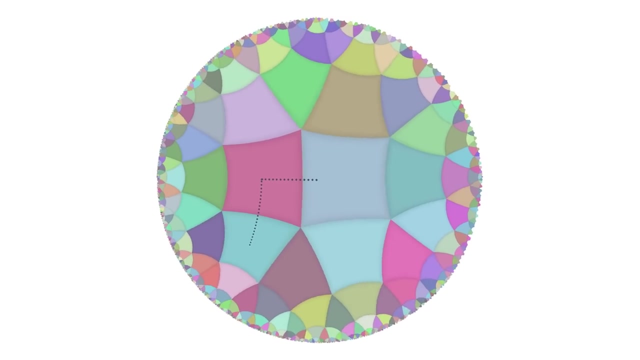 in Euclidean geometry. Basically, as you move around the space, you accumulate extra rotation, even if you never change the direction you're facing. So take a guess what happens on a hyperbolic walk. We'll walk up one tile right one tile. 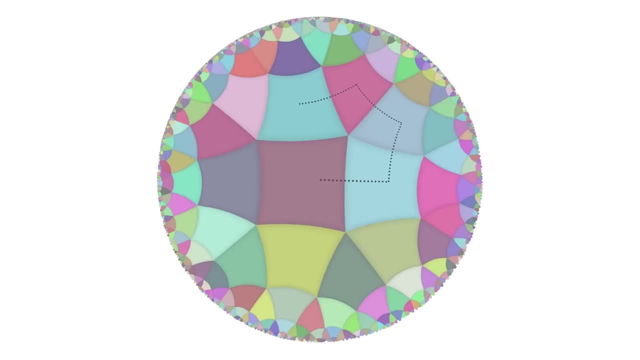 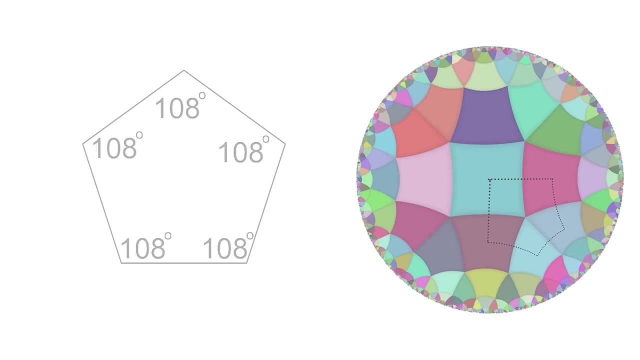 left one tile and finally up one more time. Now we've walked on a pentagon with five right angles. This time the sum is less than you would expect for a Euclidean pentagon, because polygon angles have a smaller sum in hyperbolic space than Euclidean. 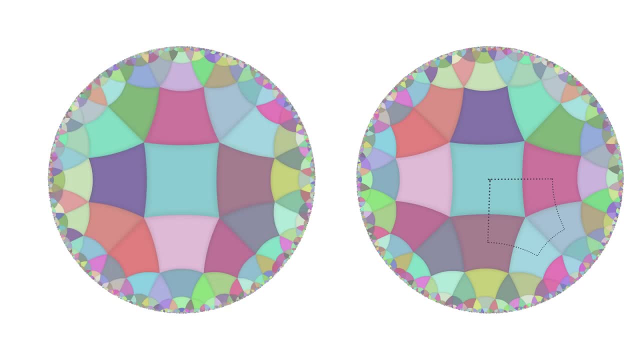 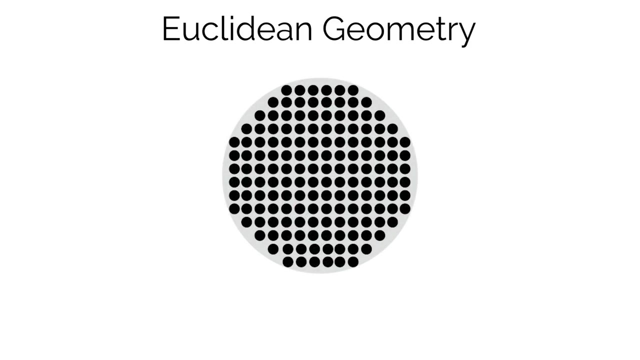 And we have the same holonomy effect, but this time rotated in the opposite direction. One last effect I want to talk about is a physical one. In the real world, objects are made up of smaller particles, and when an object moves, all of its particles move as well. 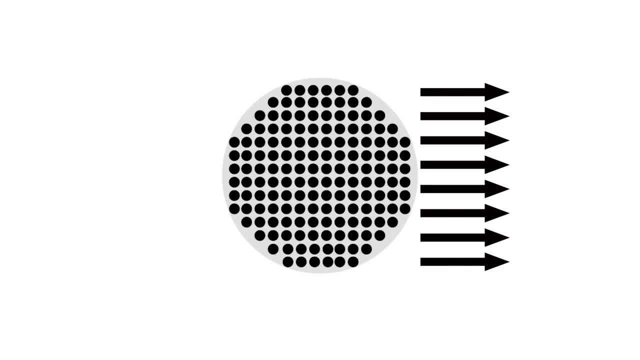 But remember, there's no parallel lines in curved space, So an object's particles can't actually all move in the same direction. In spherical geometry this means you'd experience a sort of squishing tidal force as you try to move through space. 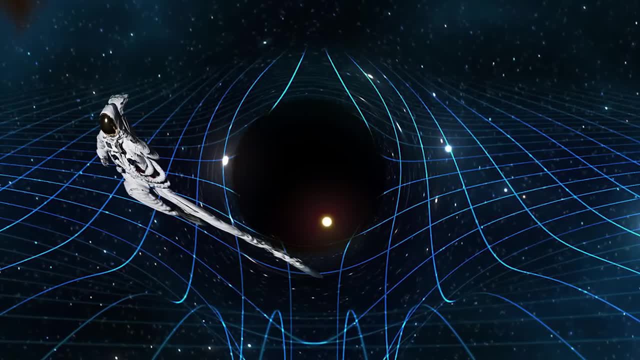 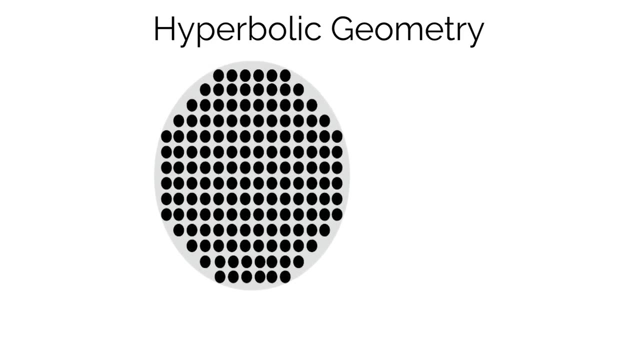 This is very similar to spaghettification around a black hole, which is also caused by curved space And in hyperbolic space, Objects experience a stretching tidal force as they move With enough speed and curvature, hitting a hyperbolic baseball could actually rip it. 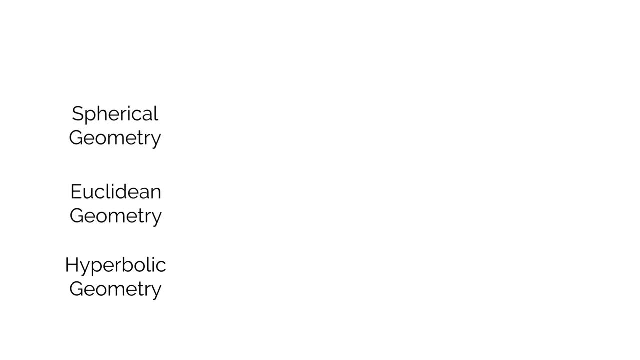 apart. Okay, let's switch over to some formulas. How would a curved space affect the circumference of a circle? It's 2 pi r in Euclidean space, but it's pi sine r in spherical space. It should kind of make sense why this is true. 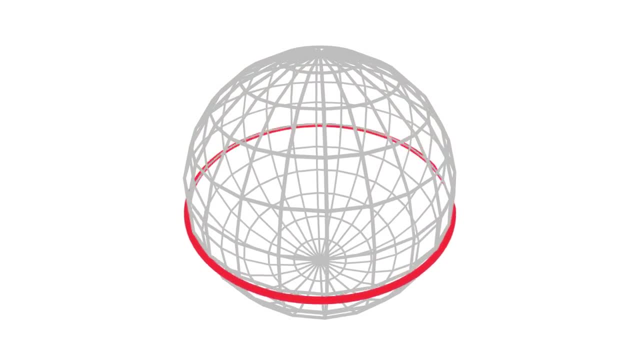 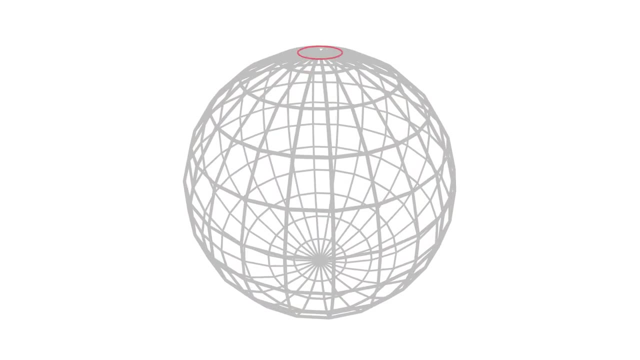 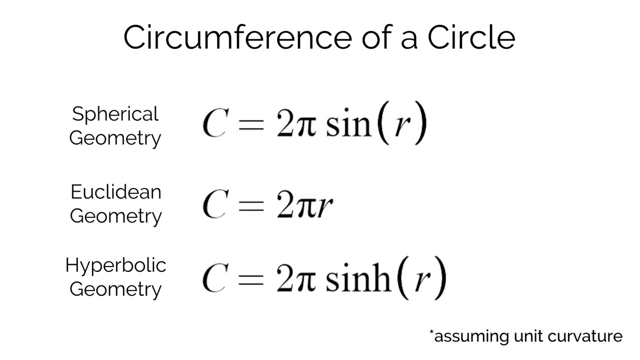 As the radius gets larger, it reaches a maximum circumference, then shrinks down to zero and repeats cyclically. Wanna guess what the hyperbolic opposite is? It's hyperbolic sine, of course. And this is another really good example of just how large hyperbolic space is, because 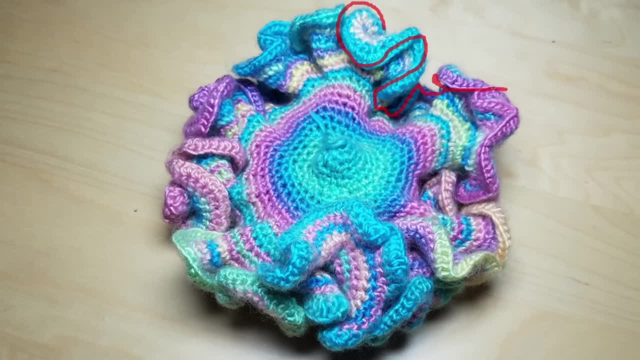 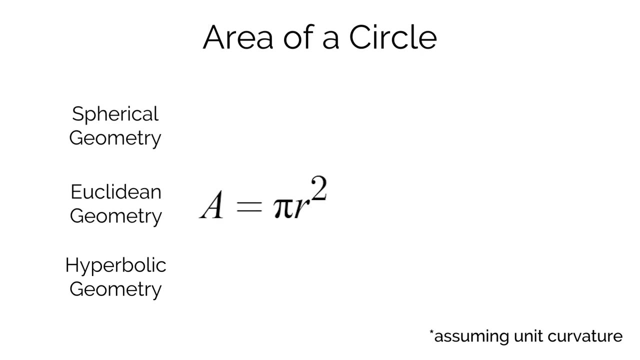 this is basically an exponential. here. That means it could take a million times longer to walk around a circle than it would to just walk across it. The area of a circle also has similar formulas. Again, area is exponential for hyperbolic space. 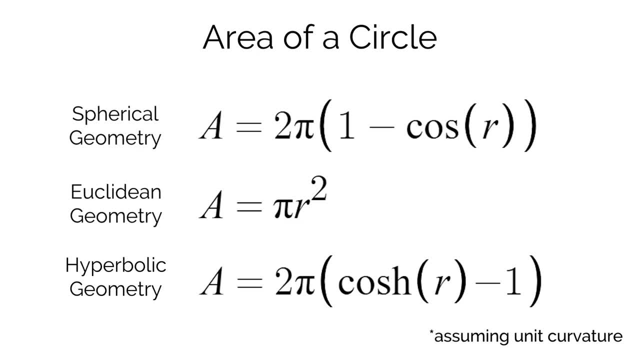 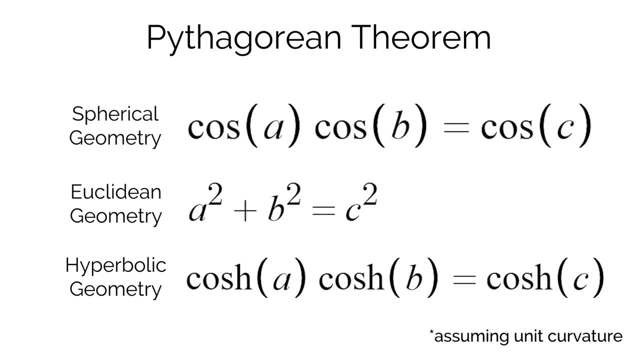 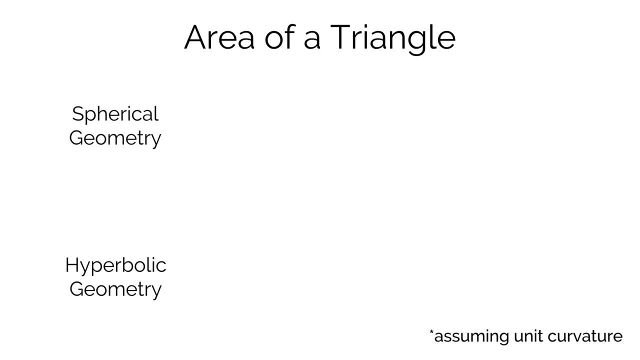 But interestingly it grows at the same rate as the circumference, unlike Euclidean space, where it grows as the square. The Pythagorean formula also has really beautiful analogs in curved space. And finally, this was one of the coolest formulas and there's no Euclidean version of it. 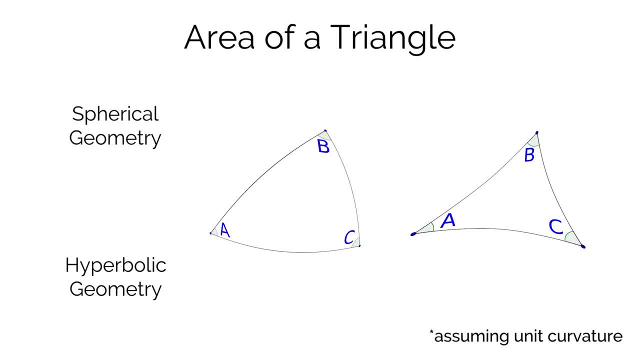 In a unit curved space, you can find the area of any triangle, given only its angles, And the formula is so simple. For spherical space, it's just the sum of the angles minus pi. That's it. In hyperbolic space, it's pi minus the sum of the angles. 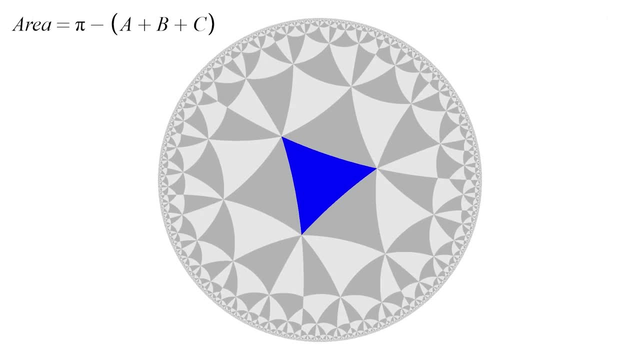 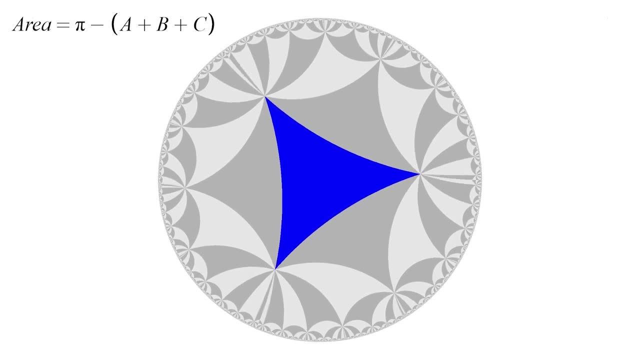 Isn't that neat. And there's a good insight from this formula. Since the sum is always less than 180 degrees in hyperbolic space, it means there's actually a maximum possible area a triangle can have, And that's when all the angles are zero degrees and the area is pi. 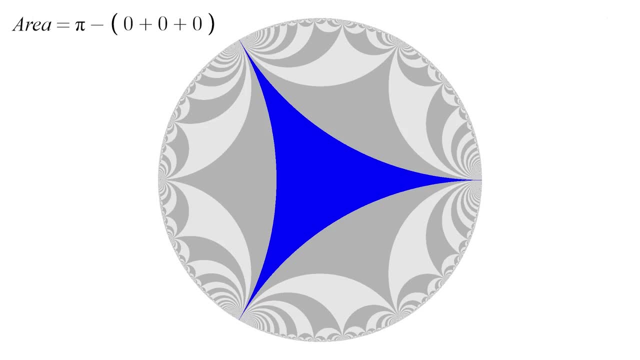 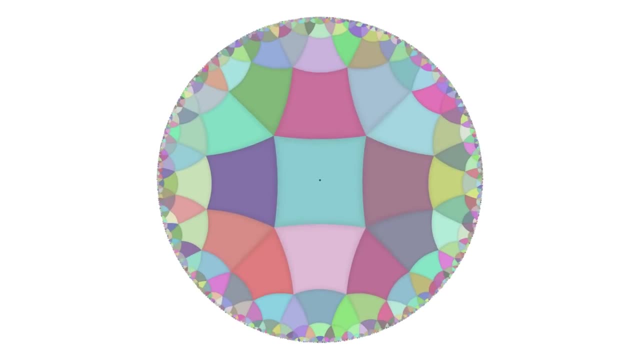 It happens because all lines eventually diverge. so if you tried to make the triangle any larger, the edges would never be able to intersect at a vertex. I hope that's given all of you a little better understanding of curved spaces. In the next video I'm going to talk more about three-dimensional spaces, how I'm able. 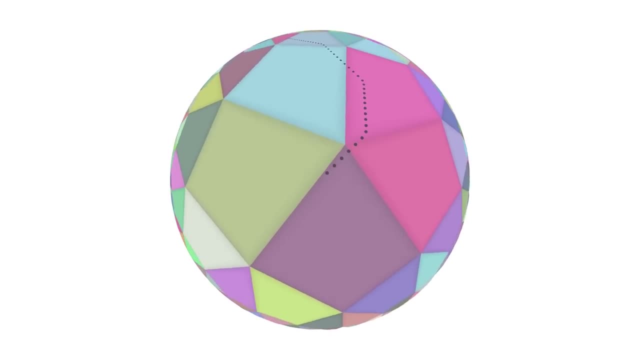 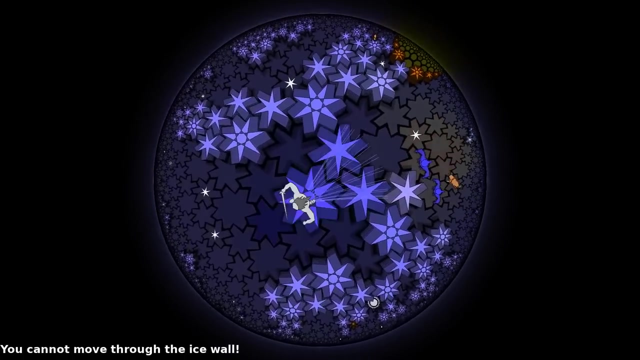 to render them in Unity and some of the really cool math behind it, If you want to build even more intuition about hyperbolic space. in the meantime, there's also HyperRogue. It's one of the only other hyperbolic games out there right now and it's worth checking.